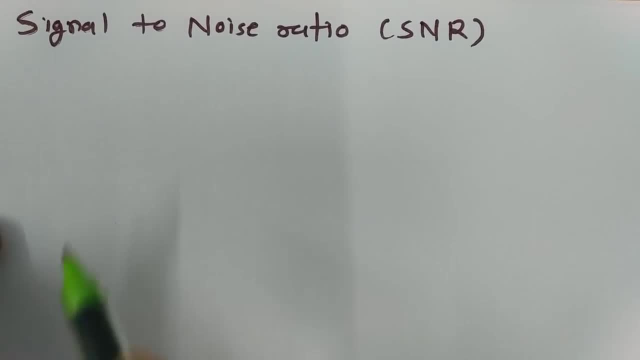 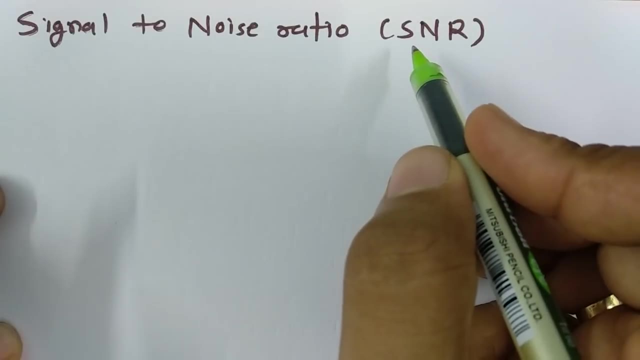 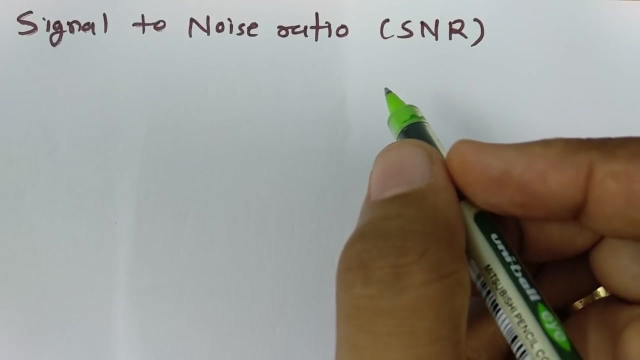 Welcome to communication engineering playlist. Here in this session I'll be going to explain signal to noise ratio. In short it is even referred as SNR. So in this session I'll explain you signal to noise ratio. Please watch till the end. The reason is I'll explain what kind of 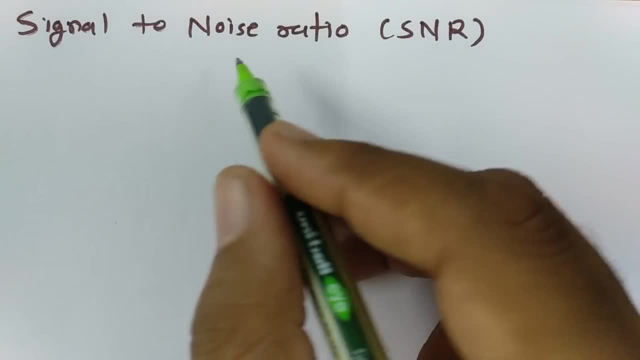 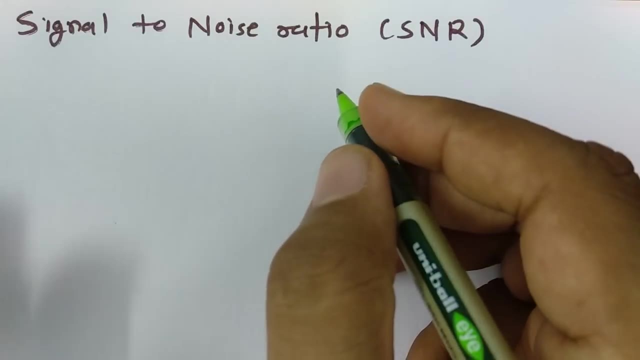 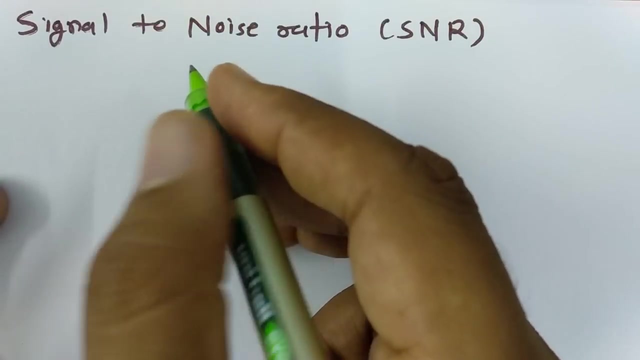 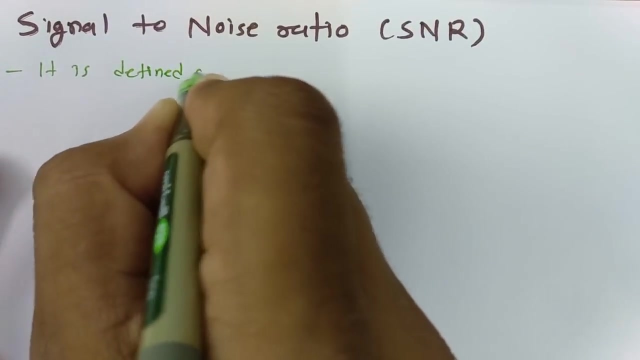 mistakes, even that students does when they calculate SNR. So when once you see this till end, it will be more clear to you. So when we talk about signal to noise ratio, it is what ratio of signal power to noise power? So it is defined as ratio. 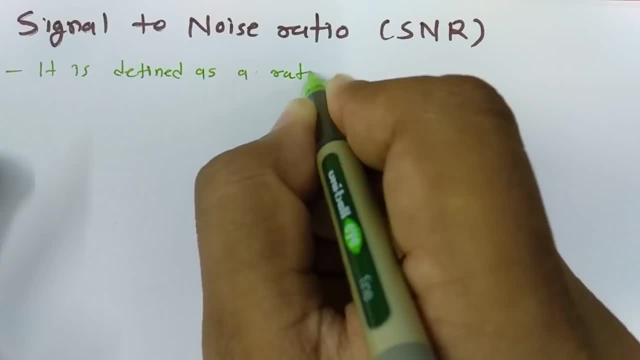 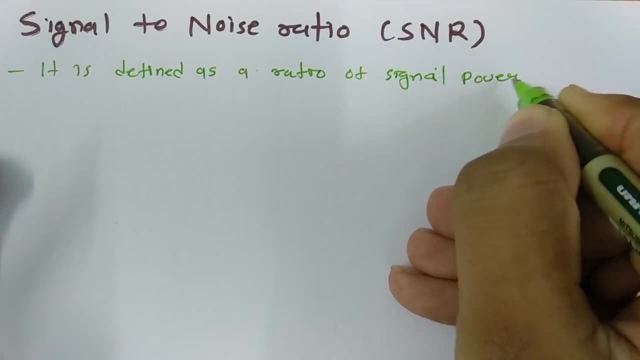 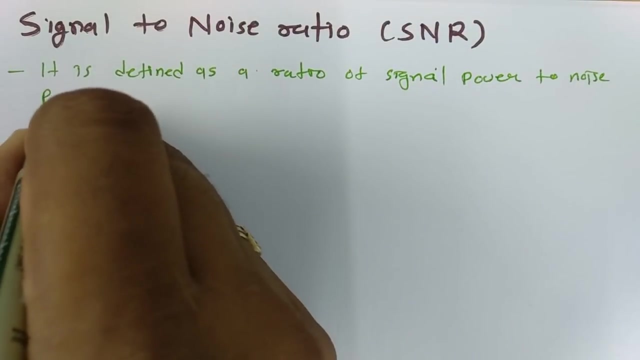 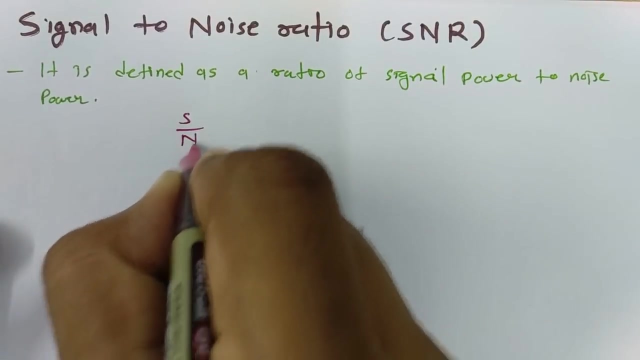 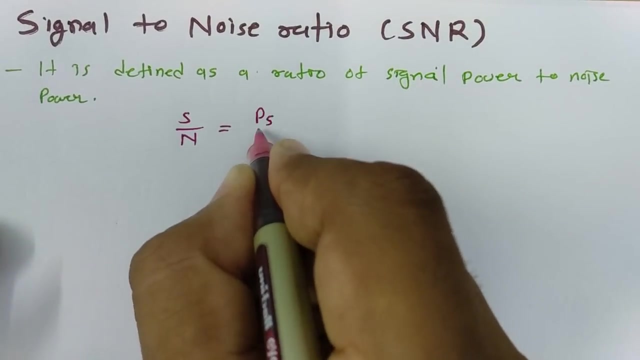 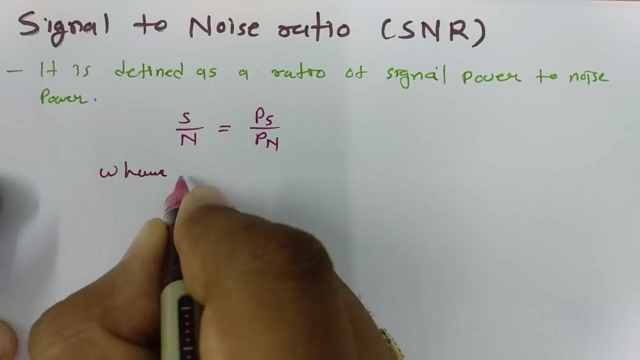 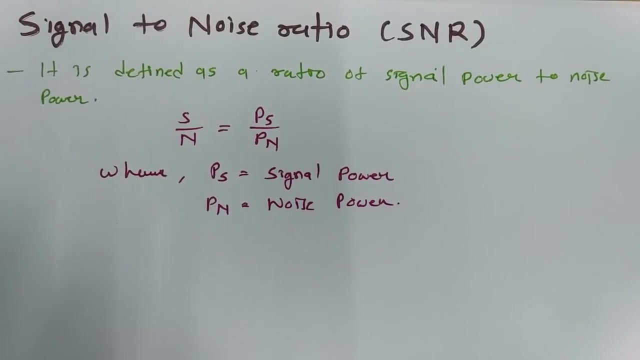 of signal power to noise power. So, basically, when we calculate this, we calculate that, as S by N means signal by noise, that is, equals to signal power divided by noise power, Where PS- that is equal to noise power divided by Señal power, and P? n, that is noise power, When we calculate, 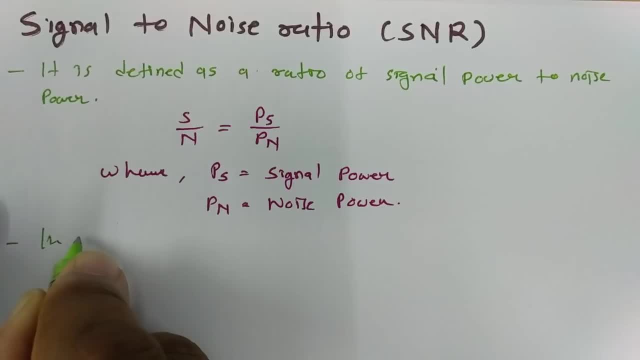 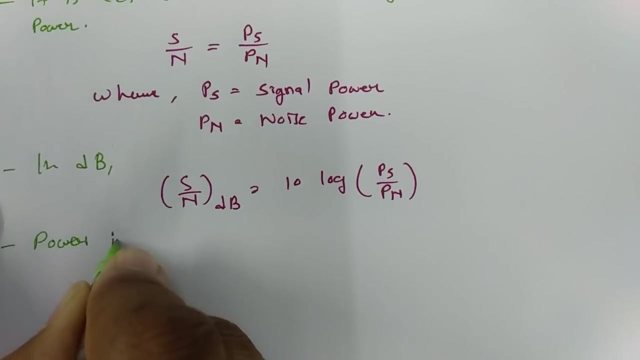 this in terms of dB. so in dB we need to take 10 log of that. So in terms of dB, SNR will be 10 log 10.. We will just add in our SNR log of PS by PN. Now we can calculate this even in terms of voltage. So power in terms. 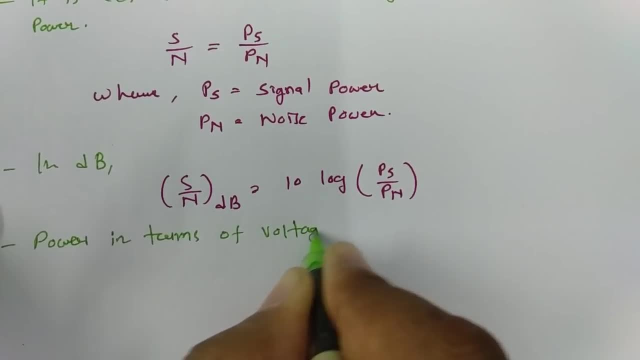 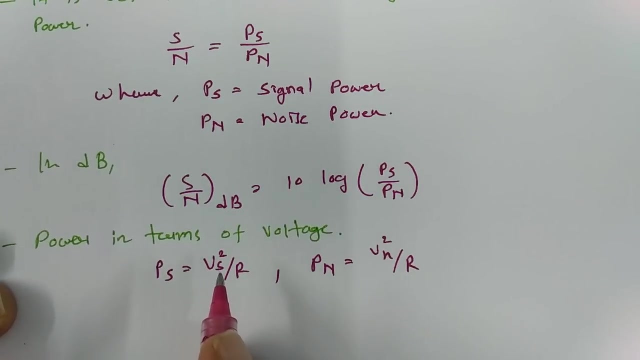 of voltage that we can calculate by signal power, that will be signal voltage square divided by resistance, R, and noise power, that will be noise voltage square divided by resistance. So V square by R. that is what power. So for signal, that will be V S square by R, where 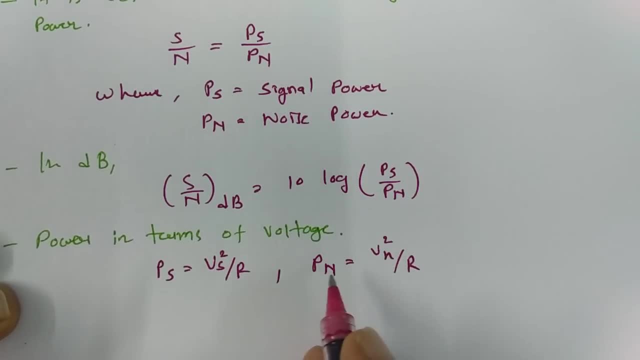 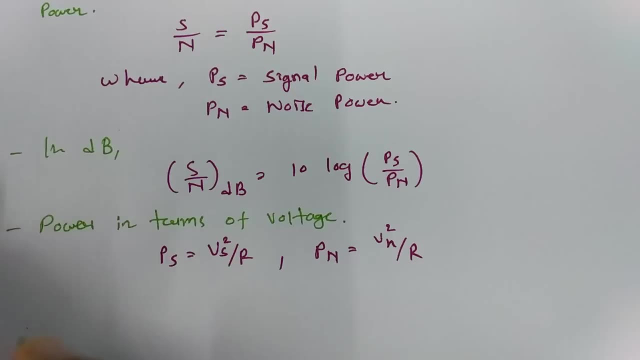 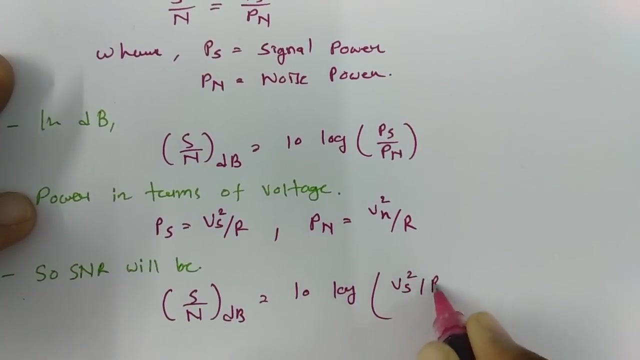 V S is signal voltage and V N, square by R, that will be noise power, where V N, that is noise voltage. So as if you place that So now SNR will be 10, log of now, just substitute this value into this, So that will be V S square. 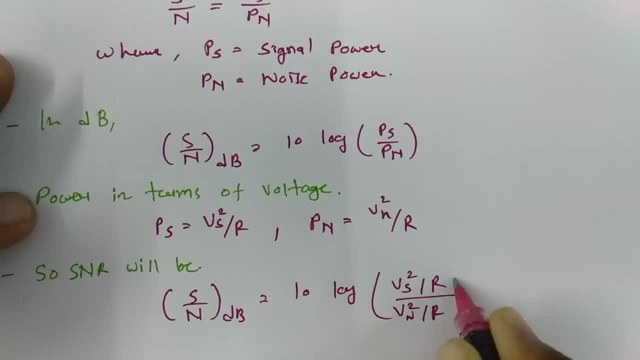 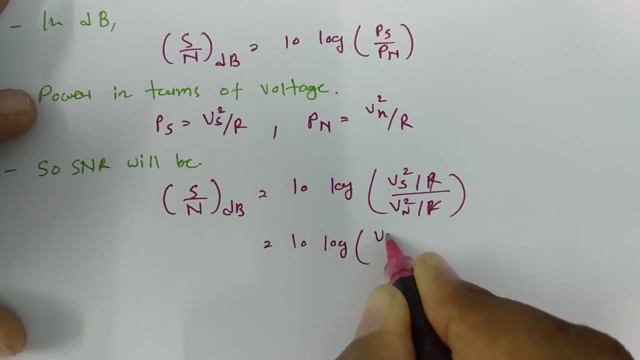 by R, divided by V? N square by R. This R, R will get cancelled, So this will be 10 log of V? S by V? N whole square. Now this square will come on front side, So this will be 20 log of V? S by V N, So SNR. 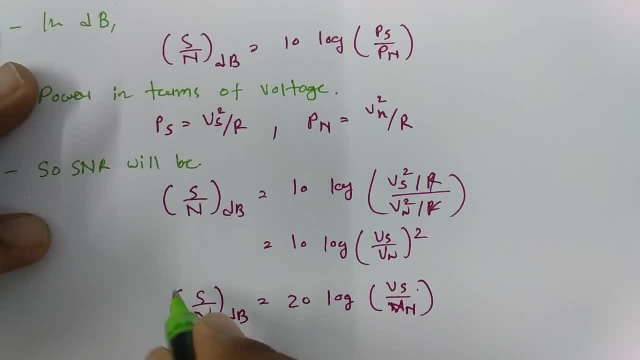 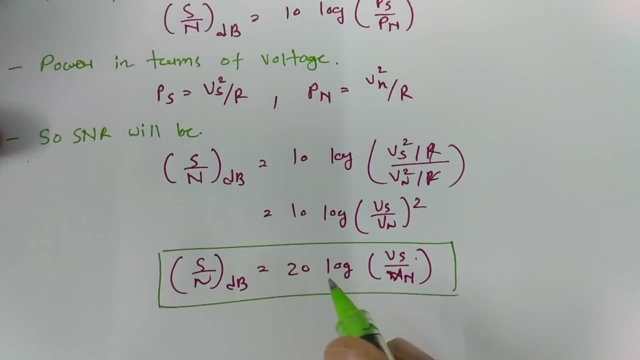 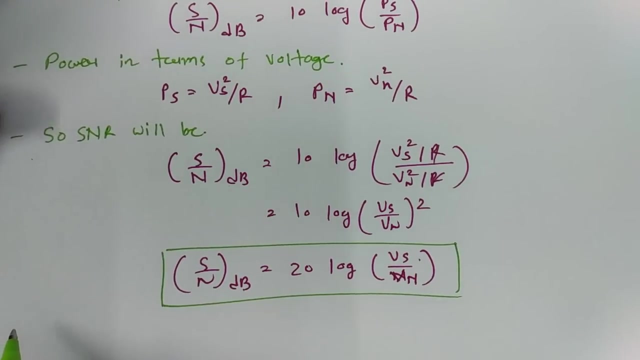 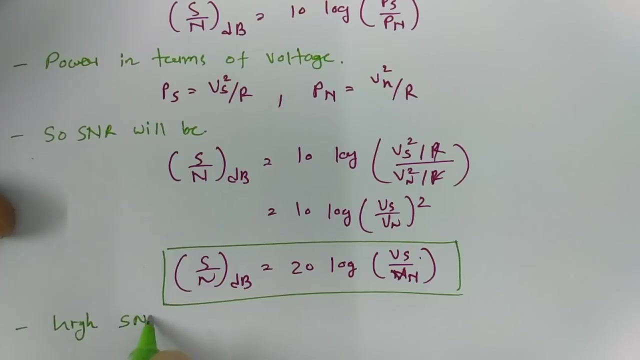 in terms of dB, in terms of voltage, that will be 20 log of V S by V? N. And one more basic that we need to understand: We should have Higher value of SNR to detect weak signal. So high value, high SNR, is good for transmitter and receiver. 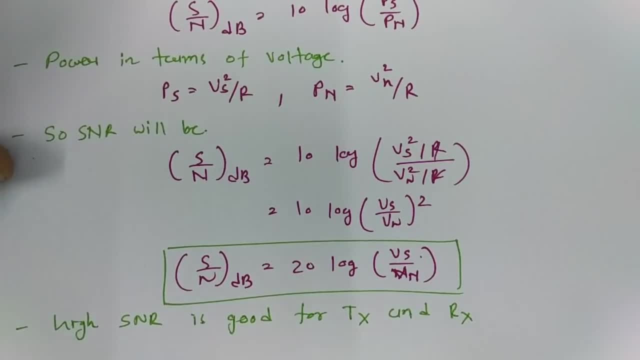 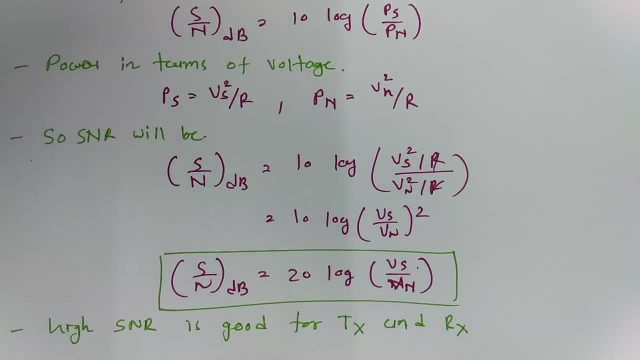 So higher value of SNR. that is good for transmitter as well as receiver. Now, as I have told you, very basic mistake Student does when they calculate SNR. See, when you calculate SNR By using voltage, at the time you should use 20 log of V S by V N. and when you calculate 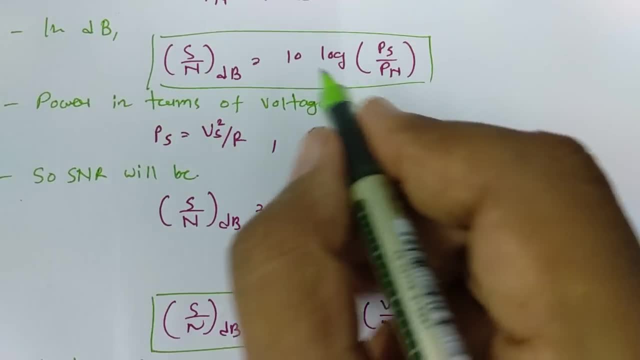 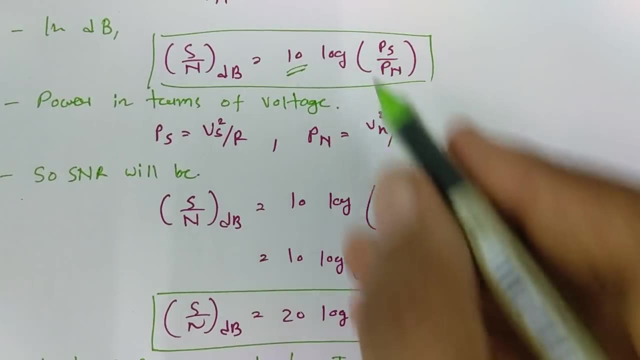 SNR by power, in terms of dB, at that time you should calculate by 10 log of P S by V? N. So this is the basic difference that is there in terms of voltage and power. So this mistake that I see students are doing. 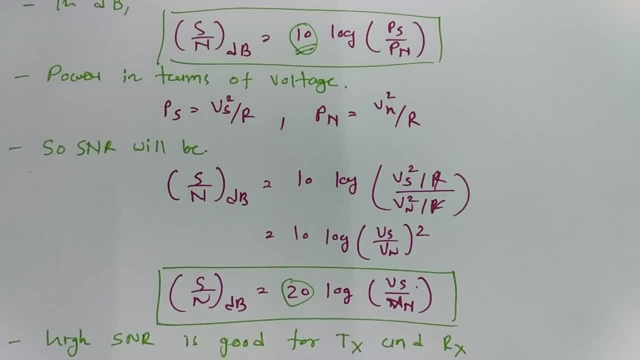 Most of the times when they calculate SNR. So when you calculate SNR in terms of power, it should be 10 log of P? S by P? N, and when you calculate SNR by using voltage, it should be 20 log of V? S by V? N.